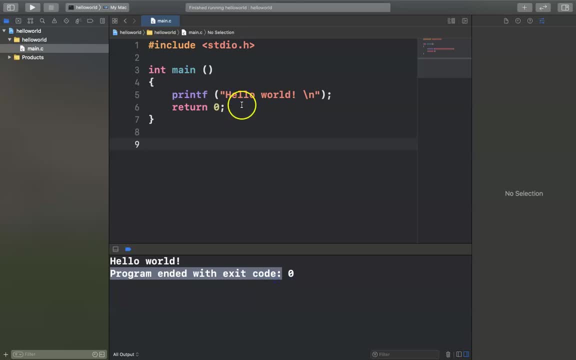 programming and with existing code 0.. So if I write more code printf here, For example welcome to cat, And then I run this again, You see the result is hello world, Welcome to cat. So you see the printf function is used for print the text like this, like hello world, Welcome to the cat. And why we? 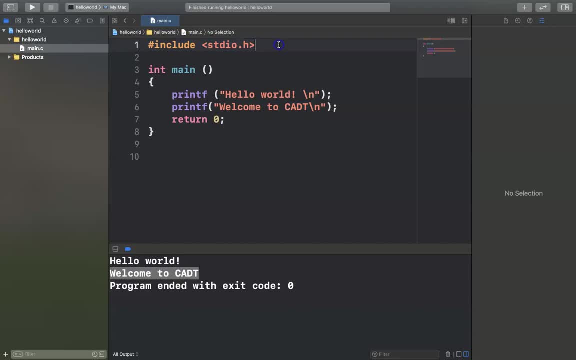 use. include stdioh. include stdioh here. stdioh is a library. You can call it a library or header file. It's up to a tutorial. Some tutorials are called library, Some tutorials are called header file. So what is the library? For example, 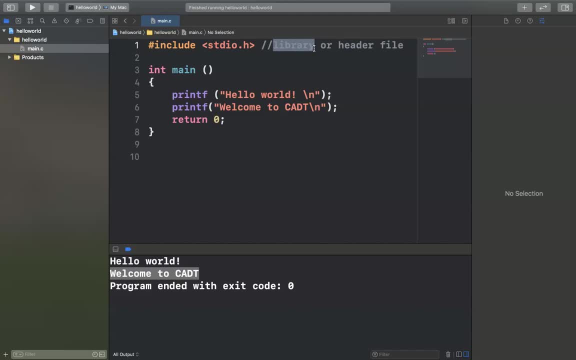 if you want to read the mathematics book, you have to go to library to access the book and then you can read it. It's similar to the C programming language. If you want to use the printf function, you have to call the library stdioh. Here include includes means: call the library stdioh, Why you have. 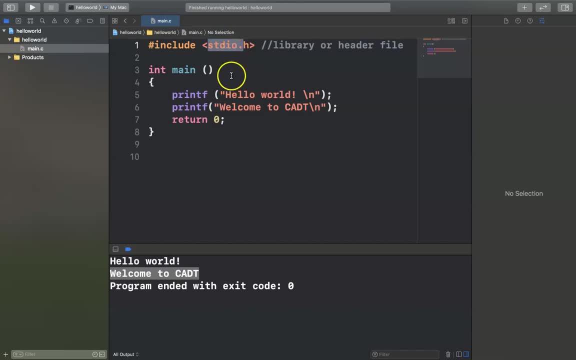 to call the stdioh, because the function printf is in the library. If you don't call the library you couldn't use the function. And then in C programming language you almost see the function main. This is: we call the function you see in main and we use a bracket And 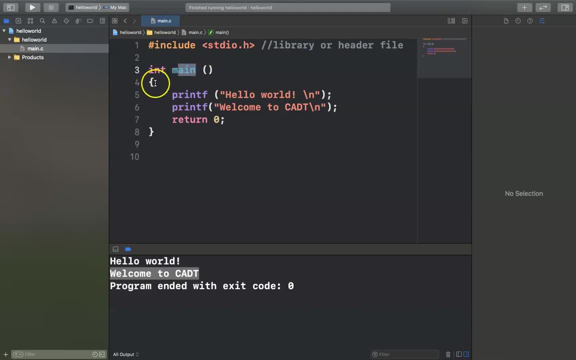 we also use a query break inside the function. Here is, here is we call the syntax In this of the function main. you can see you can write the code inside the function main. so what does the function main do? normally the code execute from the function main if in C 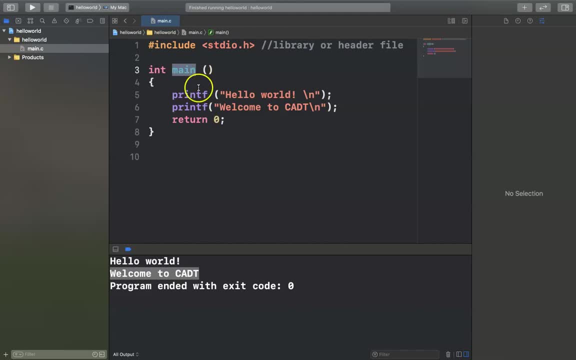 programming language. if it doesn't have function main, it it doesn't work because the code start execute inside the function main. so that why you have to create function man like this, so i can delete this one, i can remove it and i can explain you here. you see the function man. we have the tab of the function man is in in it. refer to integer. 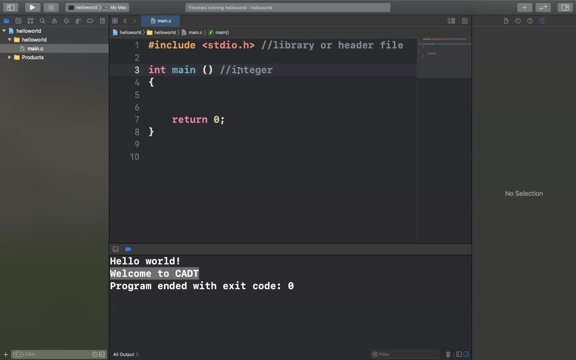 integer number. you, you know integer number. it has a lot of layer: number minus one number, zero, number one, number two and extra. it's called integer. so the function man has the tab of in here you see integer. it should finish with the code return. integer return: it means the function is finished. 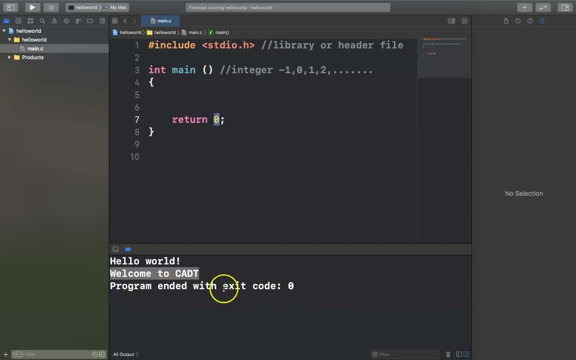 you see here program and with exist code zero here so far. so here let me run it again. you see, you see here the code with existing zero. so if i put here is two and then run again you see the code and with exit code two. so return it means that the function, if finished with the value of two, 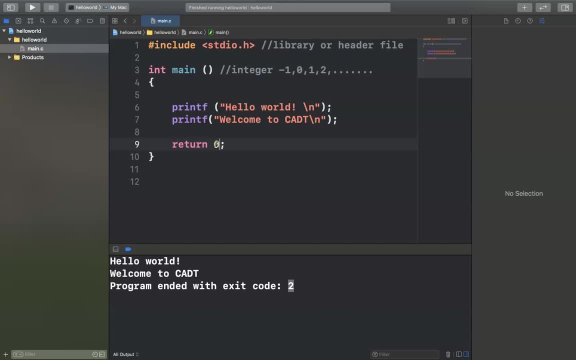 normally i recommend you to use zero. zero it means that it end, it means that the the code is end. so you can you return zero and then inside the function man you can write whatever you want here. so here we can serving you and error, network, alsoax and items like in the parameter. 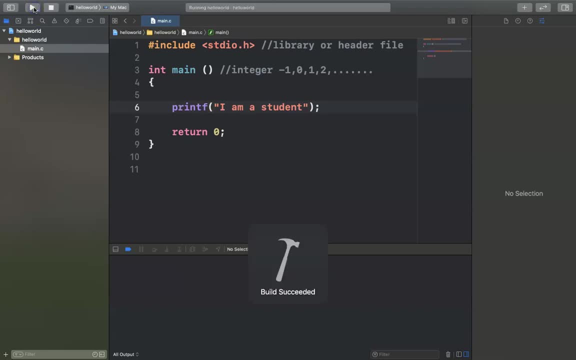 soία server waiting, no 1 chance in it. and if n, if %1 is not active, then for example we don't know our scenario. for example, in the previous command we use is table one to slash invincibleber. but when we choose exhibit forehead to save in table one, we have perspective to item four. 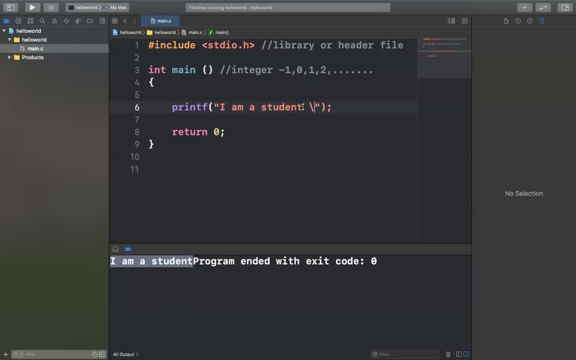 that's all relative to theítulo call sporadically to our column accurately, and so on. Then write backslash un like this and it will enter automatically when you see the backslash un You see here. So what does the backslash un mean? 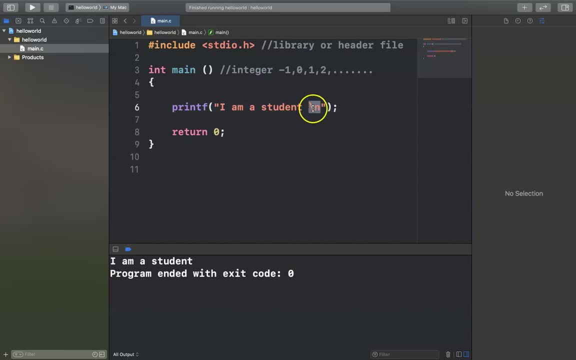 The backslash un means the new line. When you see the backslash un, it means start the new line. You also can write like this And then you will see: I am a student, thank you. And if you want to enter the new line, you can backslash un. 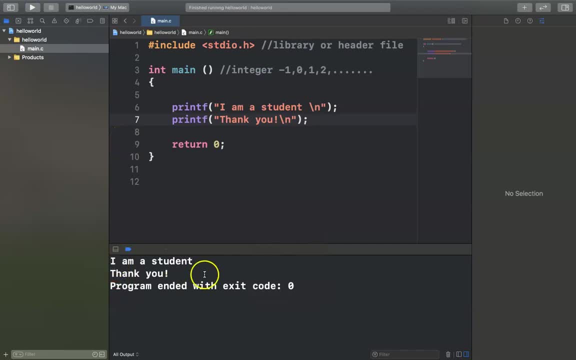 Yeah, you see, I am a student And thank you. So here is the basic syntax of C programming: language Syntax. Syntax is a rule of coding. If you write wrong syntax it means the whole of the coding will not work. 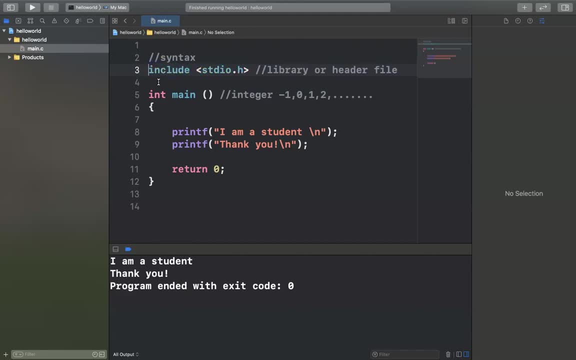 It will error. For example this one: you delete the half and it's wrong syntax. So if you run it, you will see the error. It will fail. You see It will fail. It means that it's error. So and I add the half here: 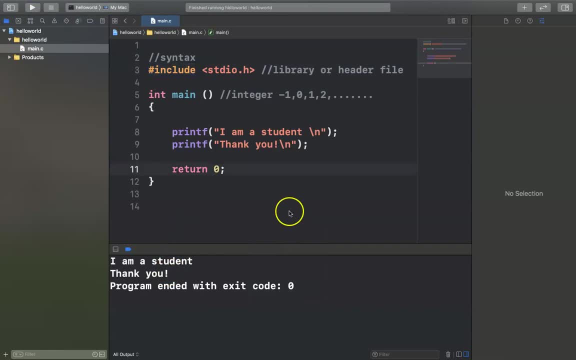 And then it correct the syntax, the code will work. So the correct syntax of main function is- let me write for you again- Correct. First you have to write the type of the function- main is integer- And then you write main. 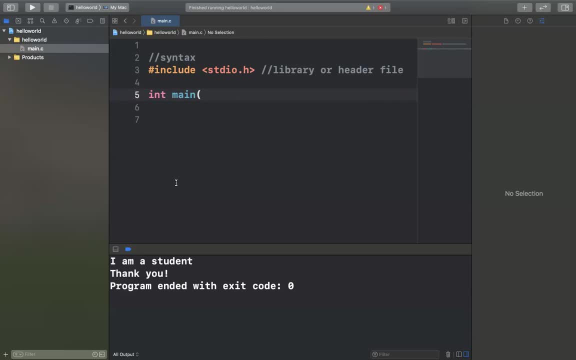 You open the brackets and close the bracket And then open the colibre And then you enter it. it will automatically close the colibre. Okay, You see, the function main is has type int, So you have to return the integer. 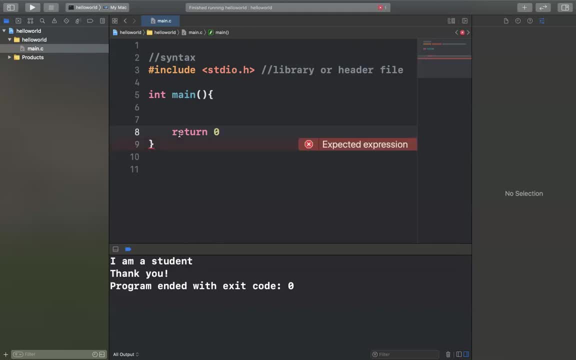 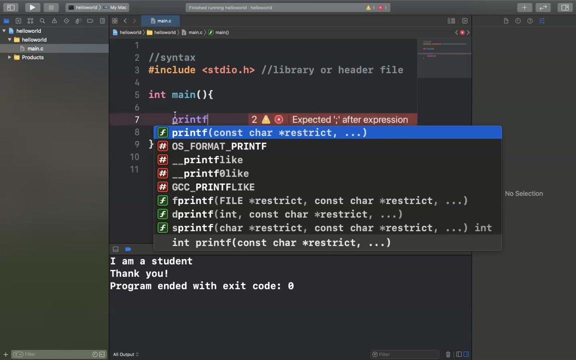 Return the integer is. you have to return zero here And then semicolon Here. you can write code whatever you want. I have to write the printf, So I can write printf, printf. The syntax of printf is printf- Open the bracket and close the bracket, and semicolon. 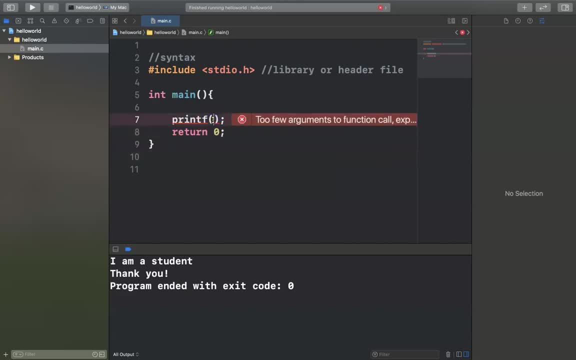 Inside the bracket you have to open the double quote and close the double quote. In the double quote you can write a text that you want to write, For example: welcome to 2CAT. Welcome to 2CAT. Welcome to 2CAT. 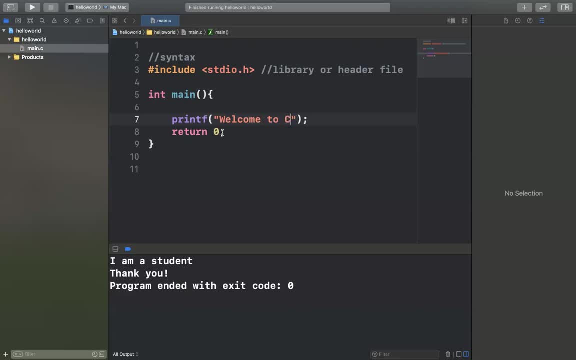 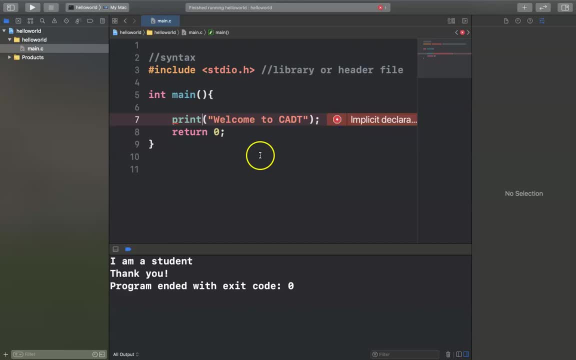 You see it's error here. If I add the f to the print it won't error. It won't solve the error. You also can use backslash n. It means newline. You have to enter to the newline to use baseline here. you can see here: welcome to cat. and it enter to the new line and you also. 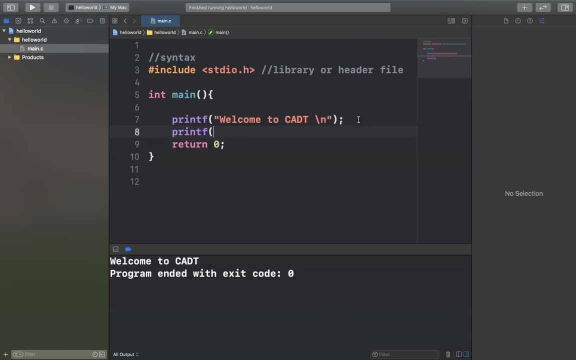 can write thank you like this: thank you and baseline and then semi column. here you see, thank you. if you don't want to use print again, you also can copy the code and you can put it here and you have to delete the code and it will output the result smf- the previous one. 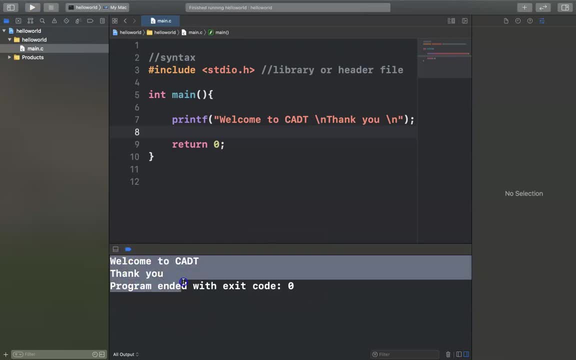 you see, here it's still the same. you can use one, only one printf function, and then it will work the same. why is it has a two line like this? because you print the welcome to cat, it's welcome to cat, and then it's meet the baseline. it means new line. 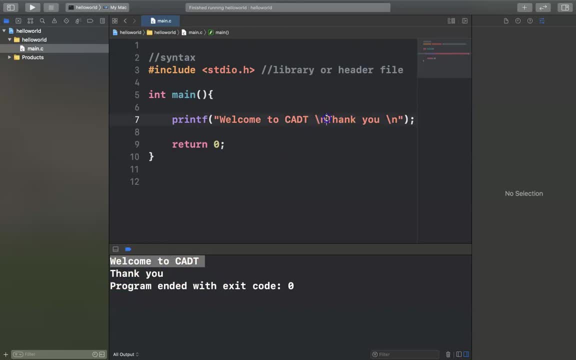 so it enter to the new line and then it meet the word thank you. it will print thank you and then it meet the baseline. it enter and then return. zero is program and with existing code zero. in c programming language you use semi column. here is called semicolon or semicolon semicolon. it means that 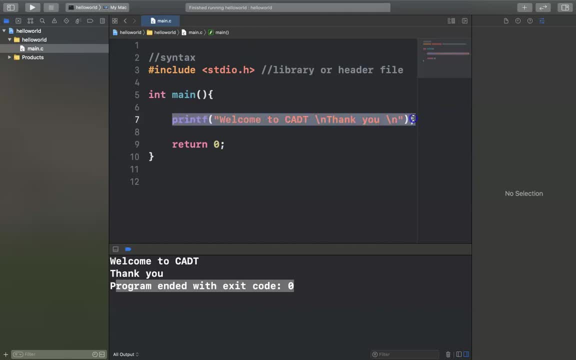 the statement of this printf function is n, and in c programming language it doesn't matter you write how many lines of code- one line, two lines, three lines or ten lines are the same. for example, here i can use only one line like this and then i run it again. 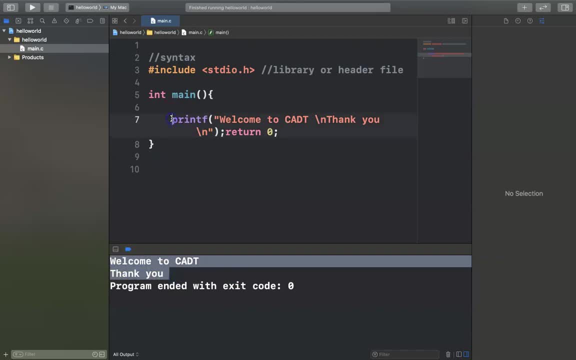 you see the same result. and also i can use one line like this. you see here is one line and like this and i print it still work. so if you write the code like this, it's very messy, it's not beauty, it's hard to understand. so you have to respect the rule of writing code. normally, if you see the function man. 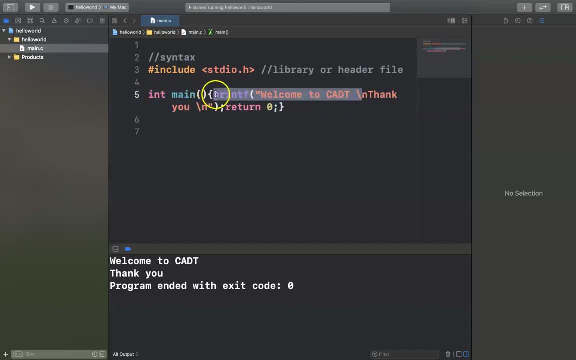 if the printf is inside the function man, it should be like this, like this: and then returns row is also like this. you see, here is the function main. start with the query break. query break. start and end cloud with the query break and you see the inside of the function. 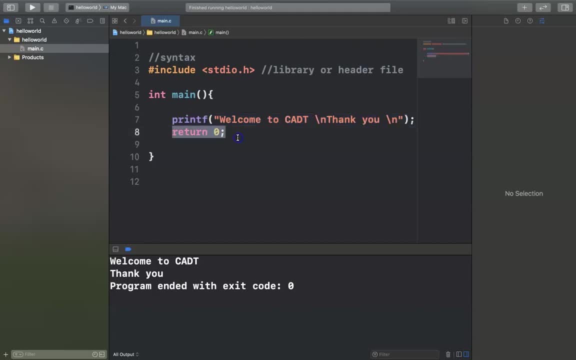 it has printf and returns row. if you don't have like this, It means that the code the same rank of the function main. So you have to tap one, tap two, tap like this. When the programmers see your code they can recognize that printf is inside the in-main.